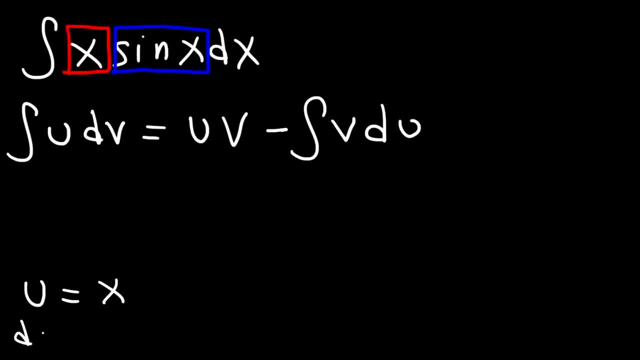 So that means that du is going to be the derivative of x, which is 1 times dx, or simply dx. Now dv is going to be sine x, with the dx as well. So if we integrate both sides, the integral of dv will give us v, and the integral of sine is negative. 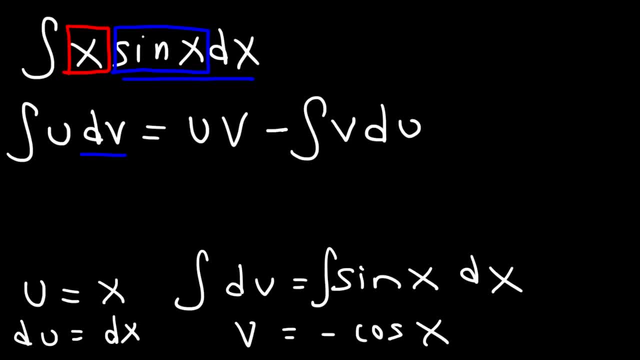 So we're going to make u equal to x, which is 1 times dx, or simply dx. So we're going to make u equal to x, which is 1 times dx, or simply dx. So we're going to make u equal to x, which is 1 times dx, or simply dx. 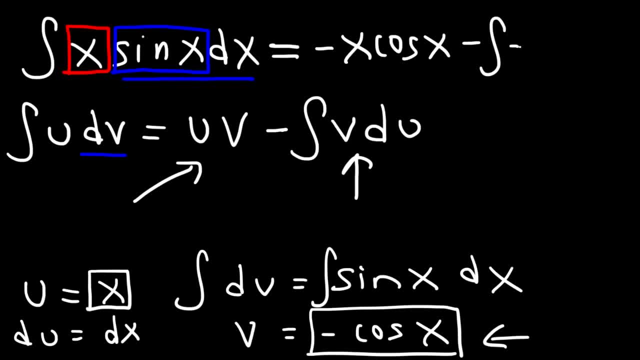 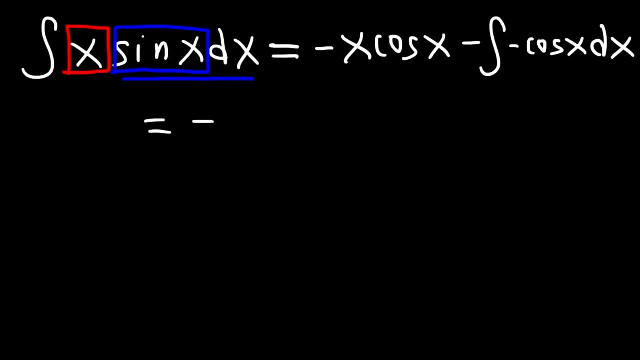 So v is still negative cosine x and du is equal to dx. So at this point we no longer need this information. So let's go ahead and get rid of that And let's simplify the expression that we now have. So we have two negative signs which we can make that a positive sign. 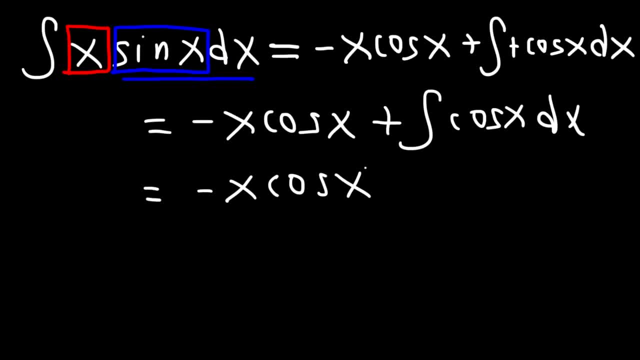 And the antiderivative of cosine x. We know it's sine x And, of course, any time you have an indefinite integral, you need to include the constant of integration plus c. So this is the answer: It's negative x, cosine x plus sine x plus c. 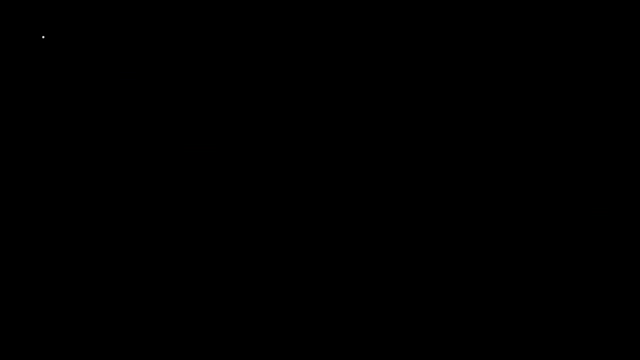 And that's it. Now let's try another example. using integration by parts, Find the antiderivative of the natural log of x times dx. Feel free to pause the video. If you want to give this problem a shot, Go ahead and try it. 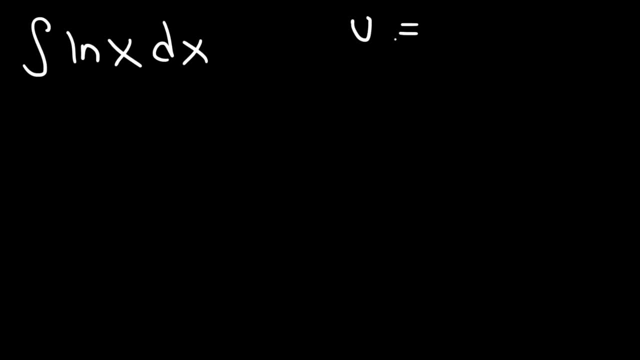 Now we need to determine what we're going to make u and dv equal to. So keep in mind the formula is: the integral of u dv is equal to u times v minus the integral of v du. So there's two parts here. 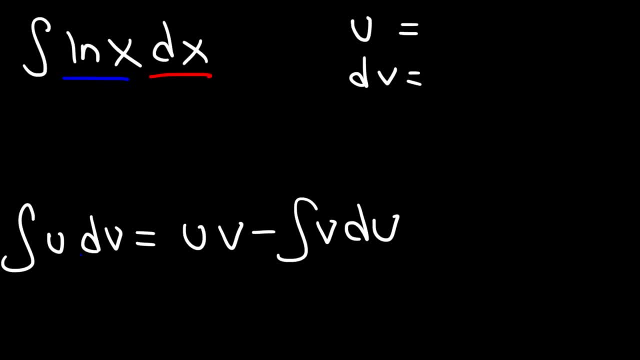 We have dx and lnx, So what should we do in this case? Now, to find the integral of lnx is what we're trying to do, So it makes no sense to set dv equal to lnx. Instead, we need to make u equal to lnx and dv has to be equal to dx. 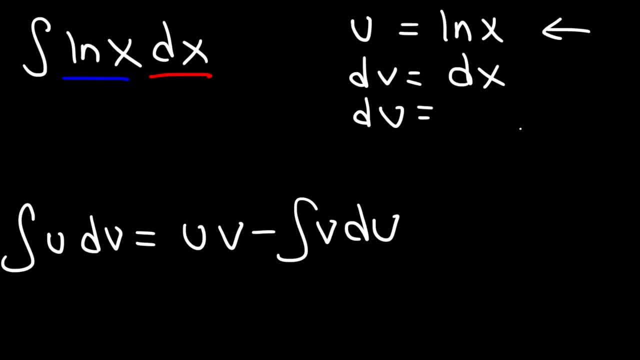 Now we need to find du. The derivative of lnx is going to be 1 over x times dx. I know this kind of looked like a v, but let me just redraw, I'm going to call that as a u. Now v is going to be the integral of dx. 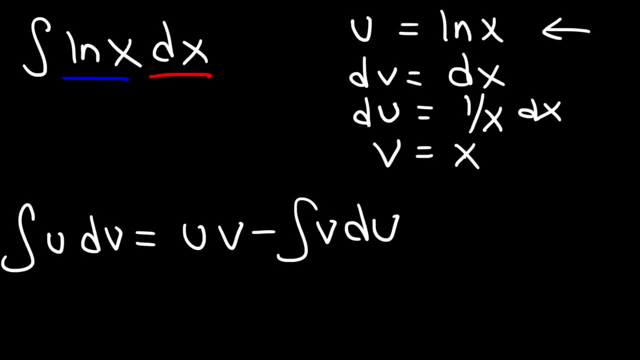 So if dv is dx, v has to be equal to x. Now let's apply the formula that we have here, So the integral of lnx dx is going to be u times v, And so we can see that u is lnx, v is x. 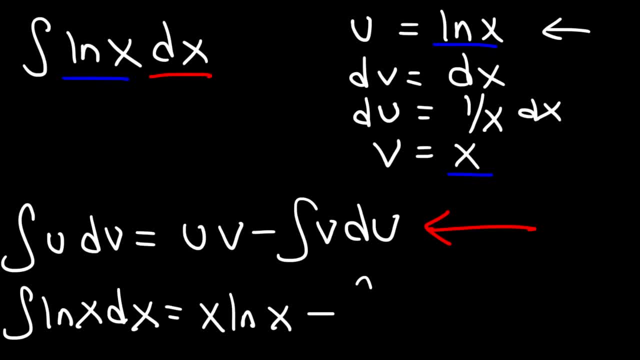 So u times v is going to be x- lnx, So we can see that u is lnx And then minus the integral of v, which is x times du, and du is 1 over x dx. So let's get rid of that. 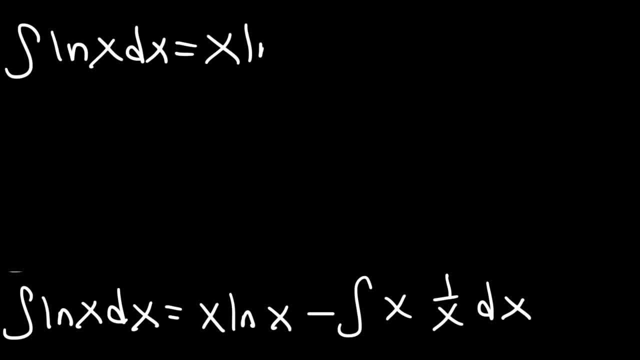 And now let's simplify the expression that we currently have. So x times 1 over x is 1.. The x variables will cancel, So we have the integral of 1 times dx, Or simply dx. The integral of dx is x. 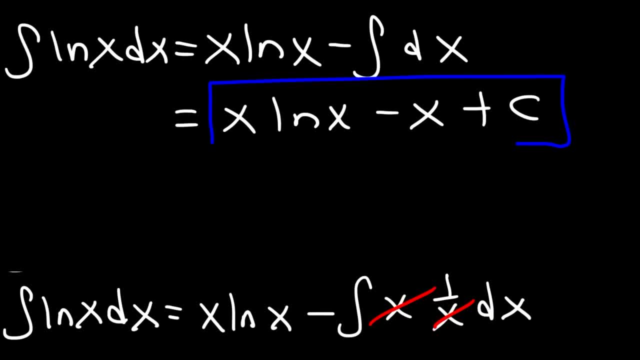 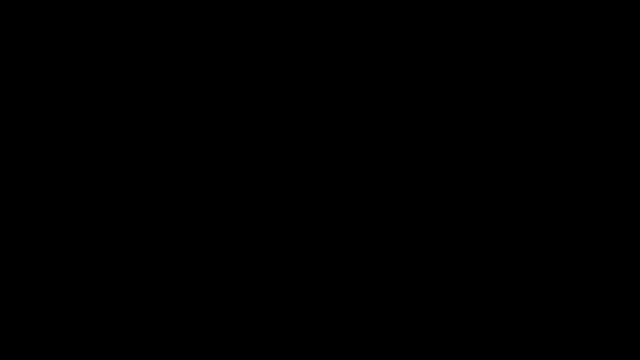 And don't forget to add plus c. So this is the answer right here. The integral of lnx is x, lnx minus x, plus c. Now the next topic we're going to go over is trigonometric integrals. So how can we find the integral of cosine cubed x, dx. 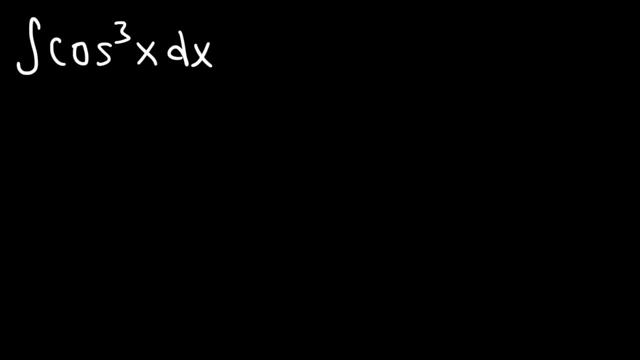 Go ahead and take a minute on that one. What do you think we need to do? So, basically, we need to do u substitution, But we need to adjust the problem that we have, For instance, cosine cubed. we can write that as cosine squared times cosine. 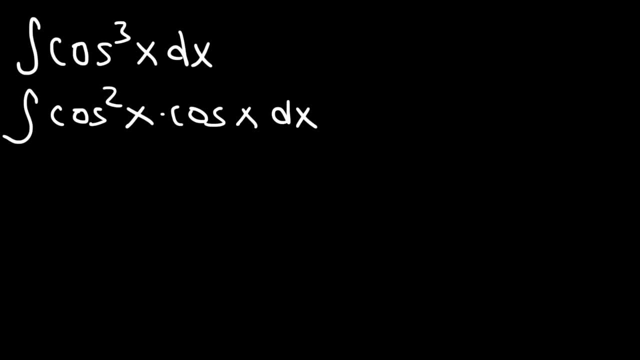 Now, if you recall one of the Pythagorean identities for trigonometry, is this one One of the Pythagorean identities? if we look at all of them individually, looks like a symbol to us. This is the one that we have to solve: forции squared. 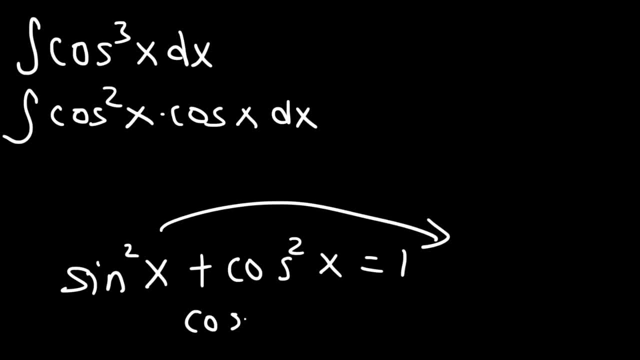 So let's back up the equation. This can be the symbol to solve for calming squared, but this can also be the symbol to cancel for symptoms. So psi squared times, sin squared plus cosine squared, And so again we're annotating a num here to prove it's a symbol to solve for the symptoms. 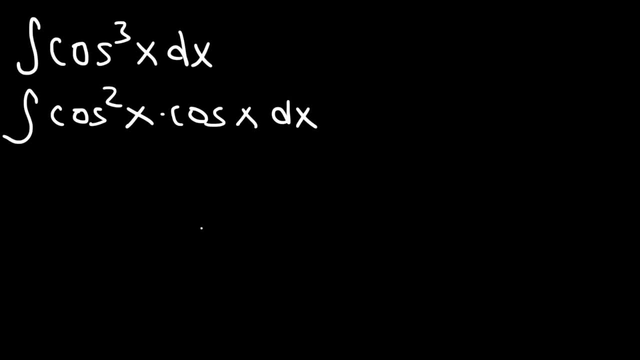 And get rid of all the fourarina ô And place the numbers here And move on to the next expression to solve for cos squared. So if you solve for cosine squared by moving sine squared to the other side, you'll find that cosine squared can be replaced with 1 minus sine squared. 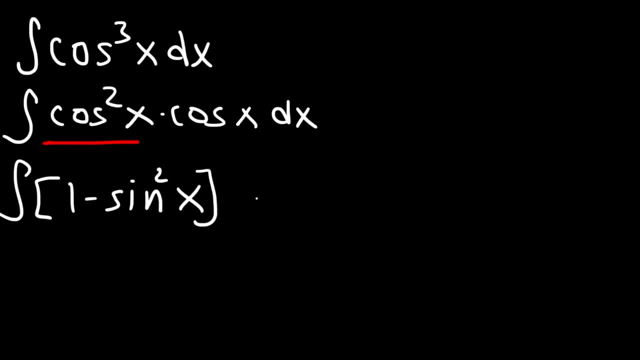 And so that's what we're going to do here. We're going to replace cosine squared with 1 minus sine squared squared times cosine. And now, in this form, we could use u-substitution. So let's make the u variable equal to sine x. If we do so, du is going to be the derivative of sine, which is: 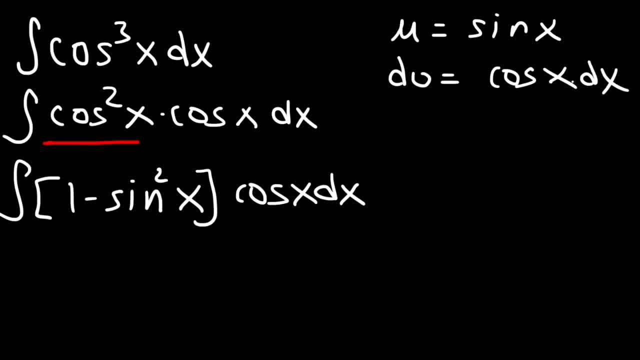 cosine x times dx. So now let's replace sine with the u variable and let's replace cosine x dx with du, And now we can integrate this. This is supposed to be u? squared, So the antiderivative of 1du is u, and the antiderivative of u? squared is u. to the third over 3, using the power rule. 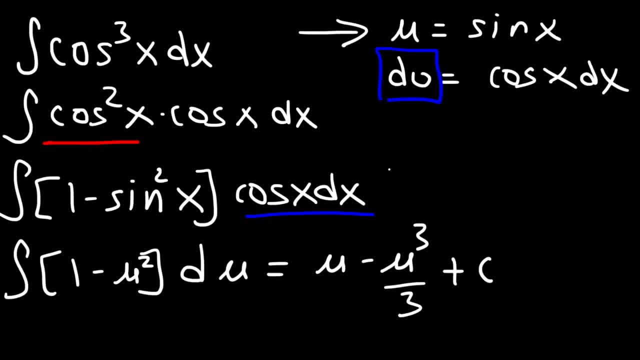 Now the last thing we need to do is replace the u variable. So the final answer: let's see if I can fit it here somewhere. Maybe I'll just have to get rid of this. The final answer is: u- squared. The final answer is u squared. So the final answer is: u squared. So the final answer is u squared. 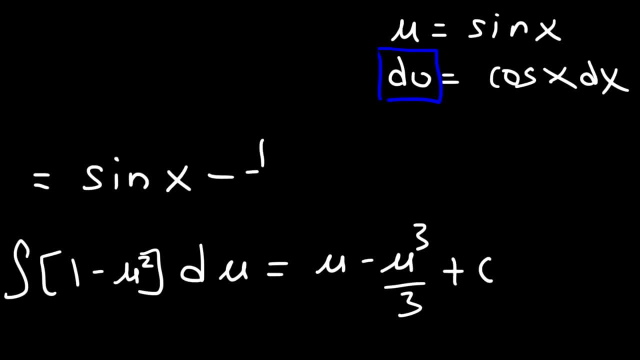 The final answer is going to be sine x minus 1, third sine cube x plus c, And that's it. That's all you need to do in this problem. Now here's another problem. Let's find the integral of cosine to the fifth power, times sine to the fourth power. So it's somewhat similar to the last problem, but it's a. 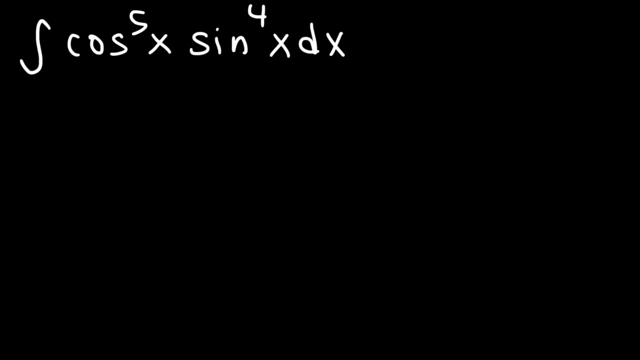 little longer. Feel free to try it if you want to Now notice that the trig function, cosine- on the left is raised to an odd power and the sine function is raised to an even power. We want to focus on cosine because it's raised to an odd power. We can split it into two components: one that's odd. 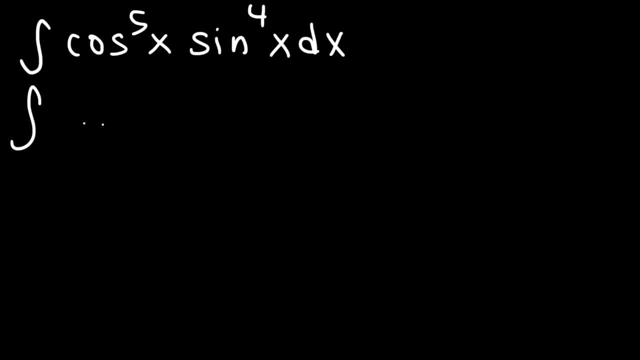 and one that's even So, cosine to the fifth power. what we want to do is break it up into cosine x times cosine to the fourth power, The even portion. we can convert it into sine, And so that's going to help us when we use u substitution. Now, the first thing we're going to do is replace cosine to the 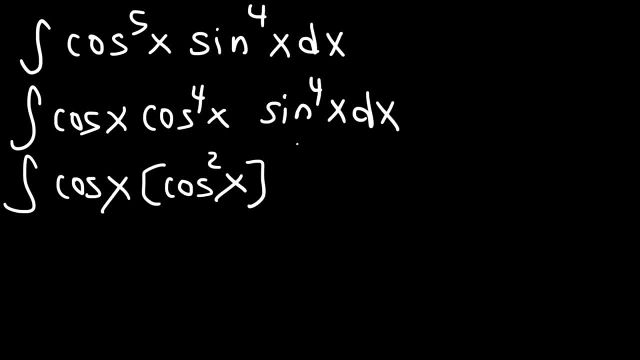 fourth, with cosine squared raised to the second power, because 2 times 2 is 4.. And now we're going to replace cosine squared with 1 minus sine squared. Now we're ready to use u substitution. So, just like before, we're going to make u equal to sine x and du is going to be cosine x- dx. So everywhere we see, 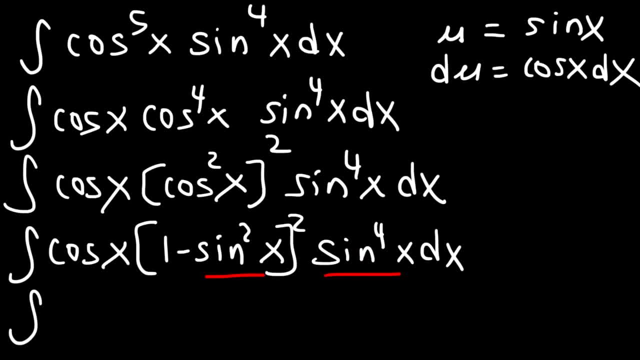 a sine function, let's replace it with the u variable. So this is going to be 1 minus u, squared raised to the second, power times u to the fourth, and then cosine x times dx. All of that we can replace with du. 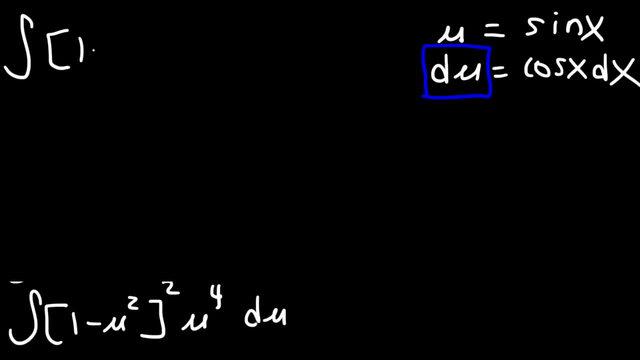 So now, at this point, what we need to do is FOIL this expression. So let's multiply 1 minus u, squared by itself, before we distribute the u to the fourth, And so 1 times 1, that's going to be 1.. And then we 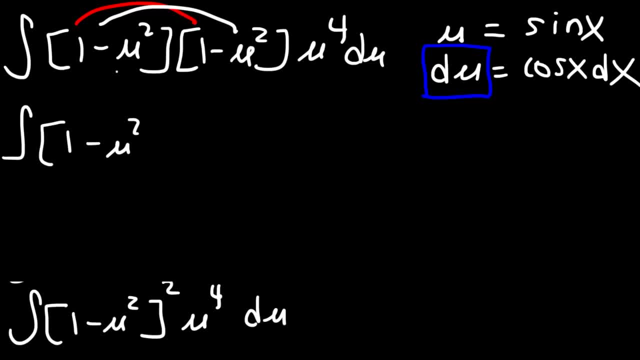 have 1 times negative u squared, and then negative u squared times 1, and finally negative u squared times negative u squared, which is positive u to the fourth. Now our next step is to combine like terms: Negative u squared minus u squared. that's going to 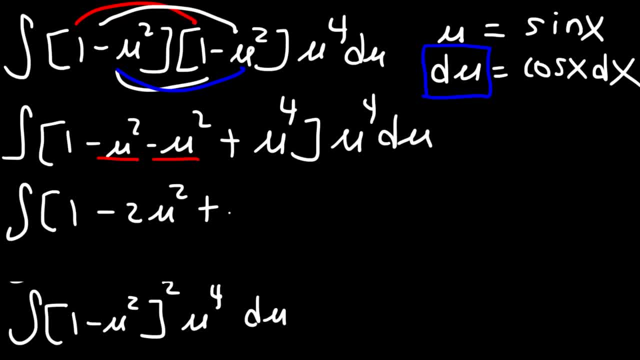 be negative: 2 u squared. Now let's delete this and let's distribute the? u to the fourth to everything inside the brackets. So u to the fourth times 1 will be the same thing, and then u to the fourth times negative: 2 u squared. 2 plus 4 is 6, and 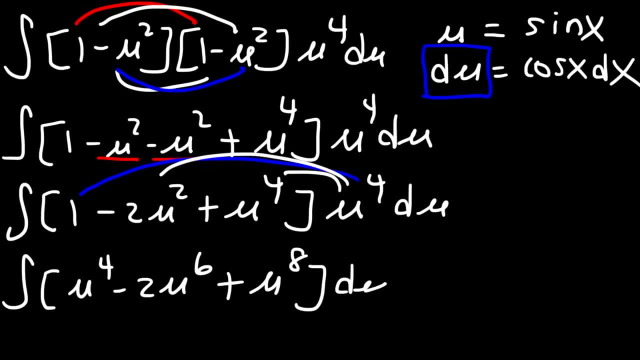 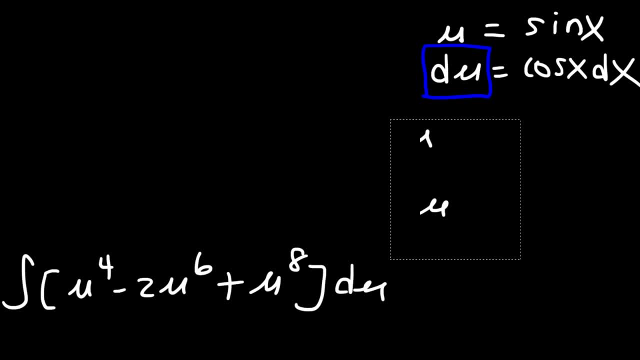 then 4 plus 4 is 8.. Now let's use the power rule in the next step. So it's going to be u to the fifth over 5 minus 2, u to the 7 over 7 plus u to the 9 over 9.. 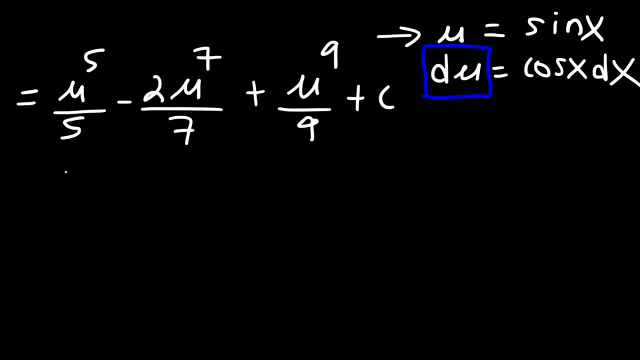 Now the last thing we need to do is replace u with sine ax. So the final answer is going to be 1 over 5, sine to the fifth ax minus 2 over 7, and then sine to the seventh ax plus 1. 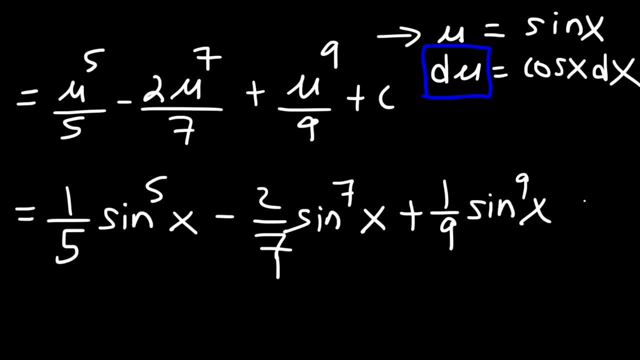 over 9 sine to the ninth ax plus C, and so that's it for this problem. by the way, for those of you who want more examples on integration by parts or trig integrals, feel free to check out my new playlist, my new calculus video playlist, and I'm gonna post the link in. 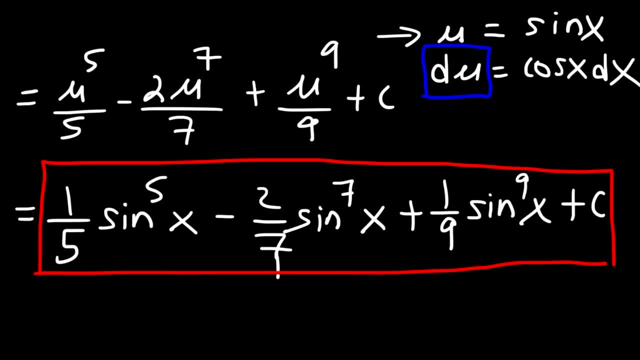 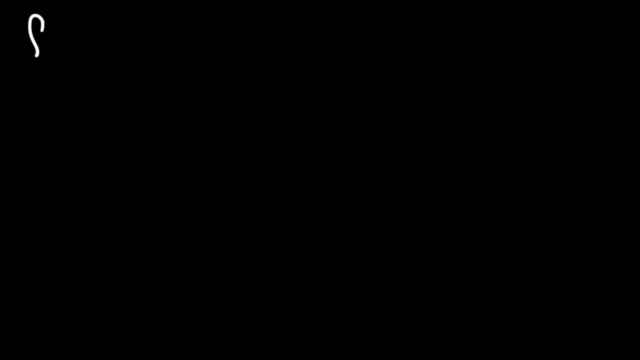 the description section so you can take a look at that when you get a chance. but in this video I'm just briefly going over the main integration techniques that you need to be familiar with in calc 2. for those of you who are going to take it now, here's another problem for you. what is the integral of sine squared? 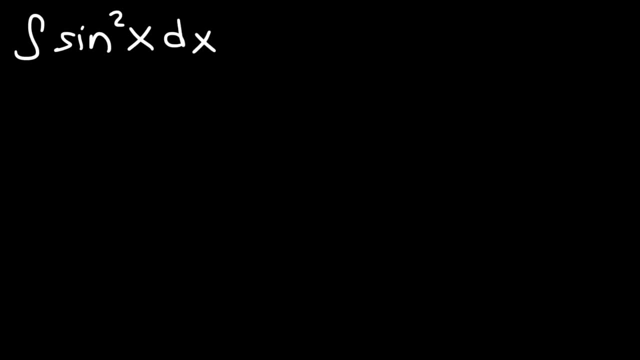 X, DX. try that one now. there's no point replacing sine squared with 1 minus cosine squared. it won't help us and this particular problem. we can't really use u-substitution, so we have to do something different, and this is where you need to know your trig identity. 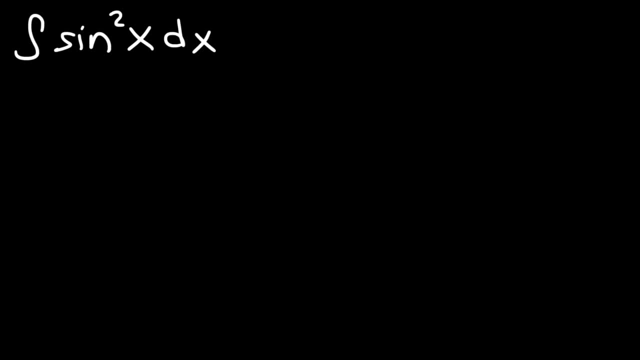 particularly the half angle identity. you need to know that sine squared is 1 half times 1 minus cosine 2x, and so we can replace sine squared with that. now we can move the one half to the front, and so we can rewrite the integral like: 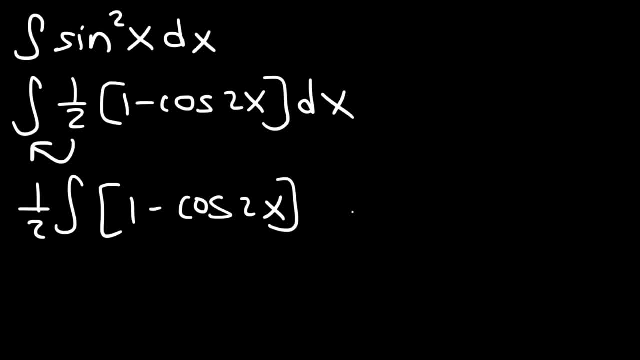 this now. at this point we can integrate the equation. so the antiderivative of 1 DX is X and the antiderivative of cosine is sine, but the antiderivative of cosine 2x is sine, 2x but divided by 2, and I'll 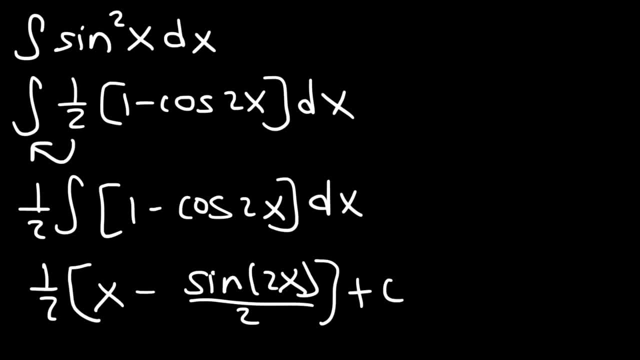 explain why, but for now let's finish this problem. so I'm going to distribute the one half, so it's going to be one half X minus, and then a half times a half, that's a fourth, or 2 times 2 is 4, so this is going to be 1 fourth sine 2x. 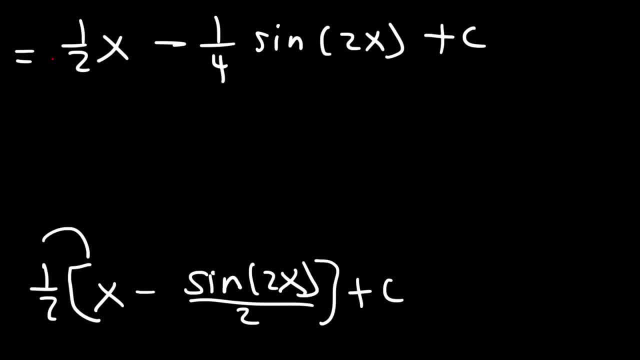 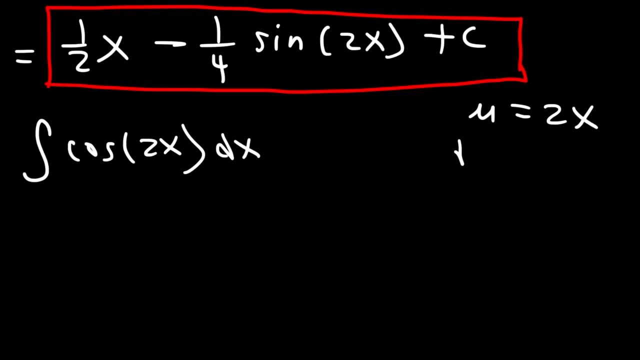 plus C, and so this is the answer for this problem. now, for those of you who want to see why the integral of cosine 2x is one half sine 2x, you need to use u-substitution. if you make u equal to 2x, du is going to be 2 times DX. solving for DX it's du. 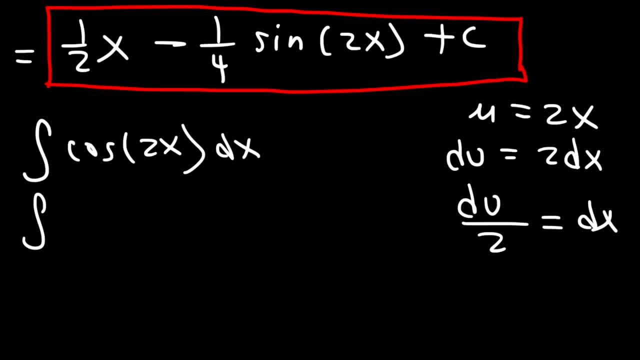 divided by 2, and so what we're going to do is we're going to replace 2x with the u variable, and so this becomes cosine of u, and then let's replace the DX with du over 2. now let's move the two to the front, so it's one half. 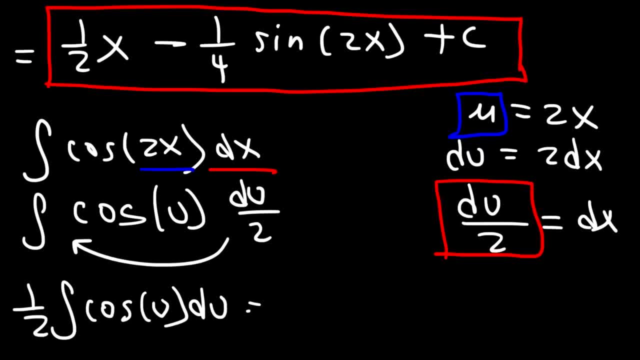 integral of cosine u. now the antiderivative of cosine is positive sine, and then the last thing we need to do is replace u with 2x, and so that gives us this answer, which is one half sine, 2x plus C, so the antiderivative of cosine 2x. 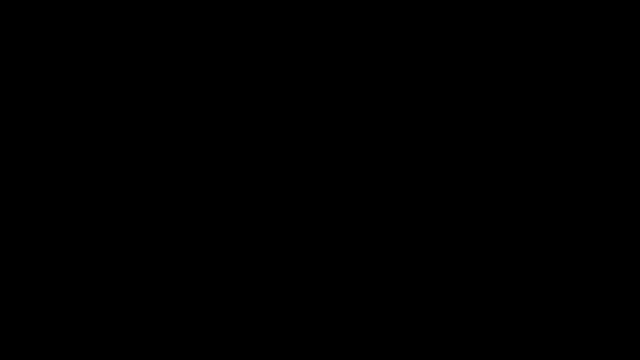 as you can see, is sine 2x divided by 2. now let's try a problem with tangent and secant. so let's try this one. let's find the antiderivative of tangent to the sixth power, times secant raised to the fourth power. now some things you want to keep in mind. the derivative of: 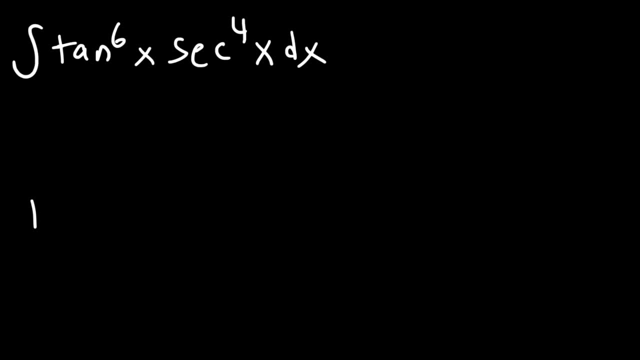 tangent is secant squared. and also make sure you know this particular trig identity: 1 plus tangent squared is secant squared. so, using that information, what is the antiderivative of tangent to the sixth power times? secant to the fourth power. now we need to make u equal to tangent, so that du is going to be secant squared. 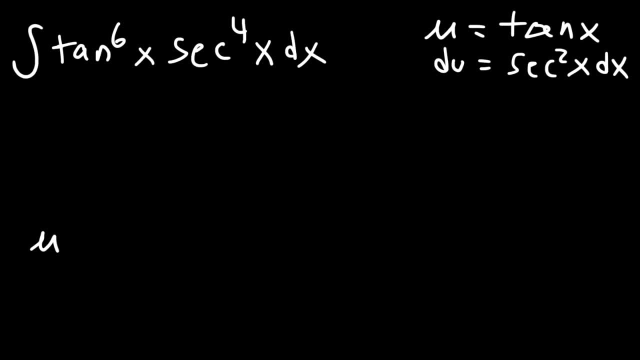 DX. if we made u equal to, let's say, secant x, du will be secant tangent, and that will make the situation a lot more complicated than it needs to be. so we're not going to do it that way. now we know that the secant squared will. 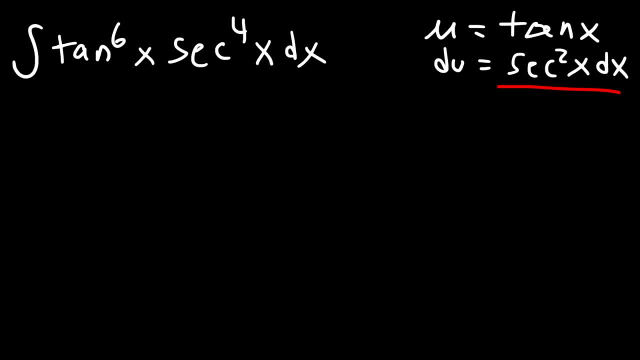 disappear, but we have secant to the fourth, so therefore we need to get rid of a secant squared in order for this to work. so let's split up secant to the fourth power into secant squared, times secant squared, so this portion secant. 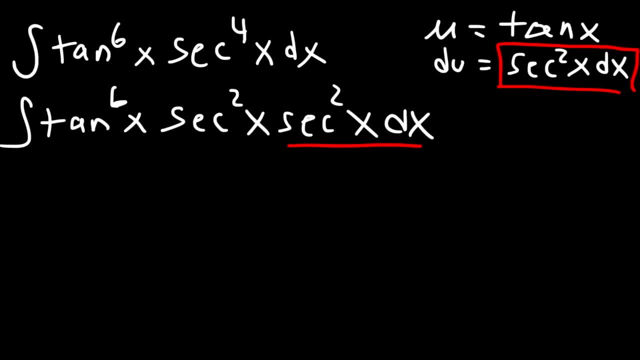 squared DX. we're going to replace it with du in time, but somehow we need to get rid of this secant squared now. recall that we said that secant squared was 1 plus tan squared, so now it's a good time to use that particular identity. so let's. 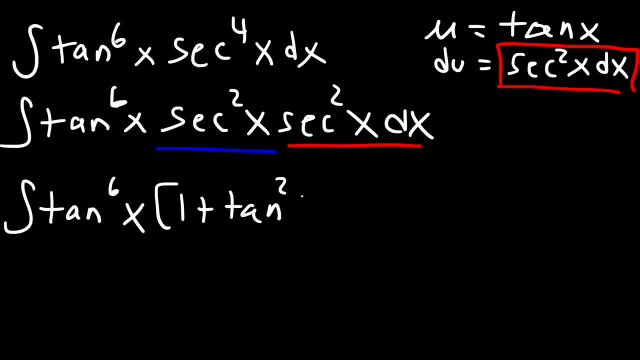 replace secant squared with 1 plus tan squared. so now, at this point, we can substitute: everywhere we see a tangent, we're going to replace it with the u variable, and wherever we see a secant squared DX, which is only here once, we're going to replace that with du. so now we need to distribute u to the 6 to. 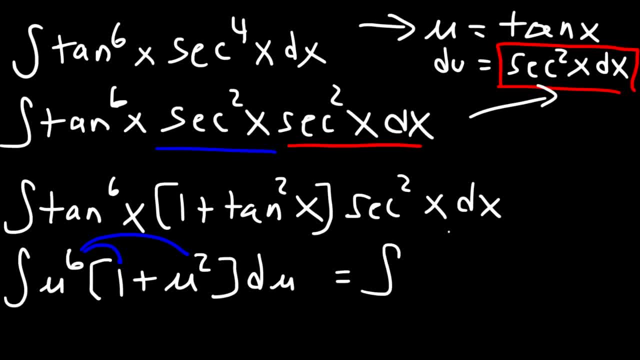 1 and u squared, so this becomes the integral of u to the 6 plus u to the 8th times hu squared. so this is our new method, and none of the library schools did it for this purposeachsenweighитьсяheut affairs. so go to the military sus. 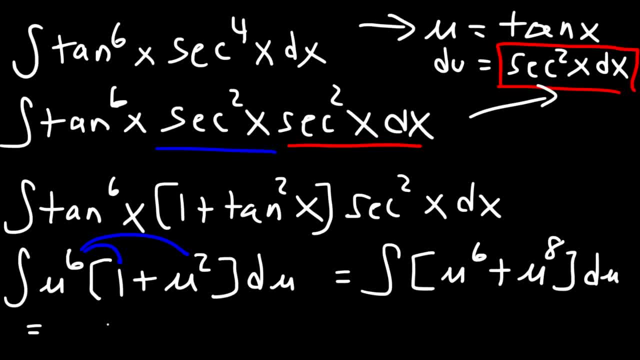 du. Now, using the power rule, the antiderivative of u to the 6 is u to the 7 over 7.. And for u to the 8, it's going to be u to the 9 over 9 plus c. So now let's replace the u variable with the. 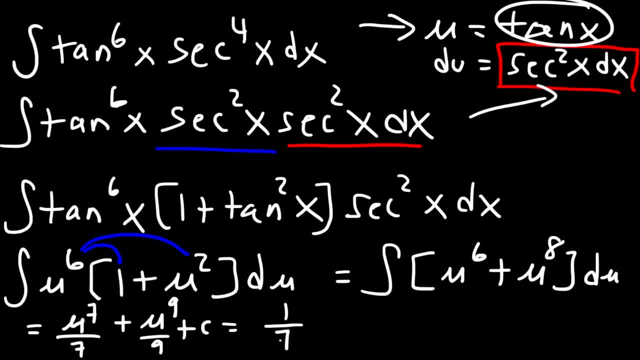 tangent, And so the final answer is going to be 1 over 7 tangent to the 7th power of x, plus 1 over 9 tan raised to the 9th power plus c, And that's it. So this is the antiderivative of tangent to. 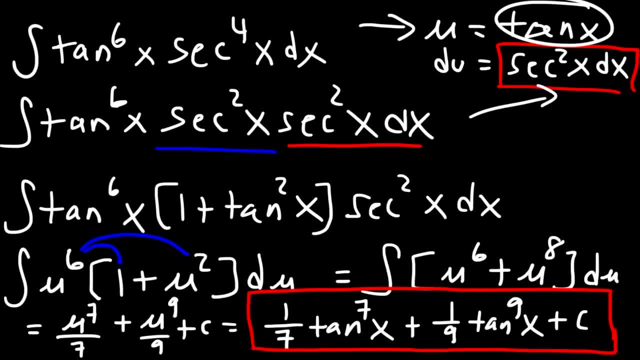 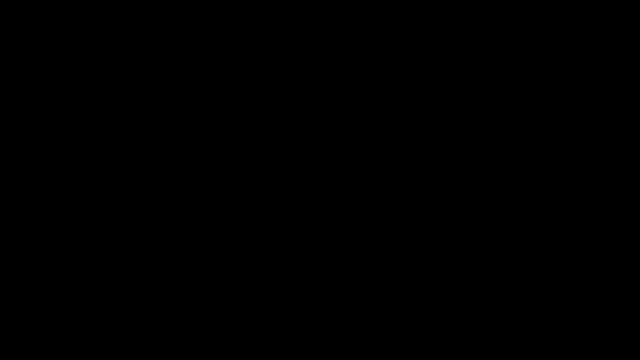 the 6th power times secant to the 4th power. Now there's something called trigonometric substitution, Another integration technique that you're going to learn in Calc 2.. And whenever you see an integration problem in this form- a squared minus x squared. 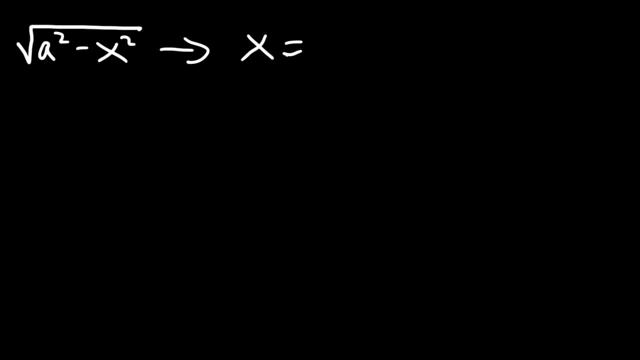 inside a square root symbol, you need to set x equal to a sine theta, And the reason for this is because 1 minus sine squared is cosine squared. If you see this form- a squared plus x squared within a root symbol, your substitution will be this: x is equal to a tangent theta And finally, 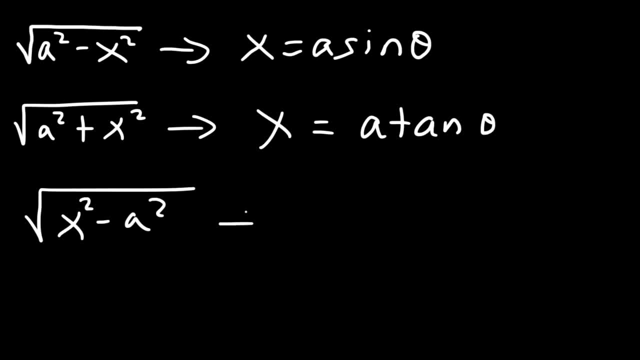 if you see the square root of x squared minus a squared, you need to set x equal to a secant theta, Because secant squared minus 1 is tan squared. So based on that, let's try a problem. Let's find the antiderivative of the square root of 4 minus x squared divided by x squared dx. 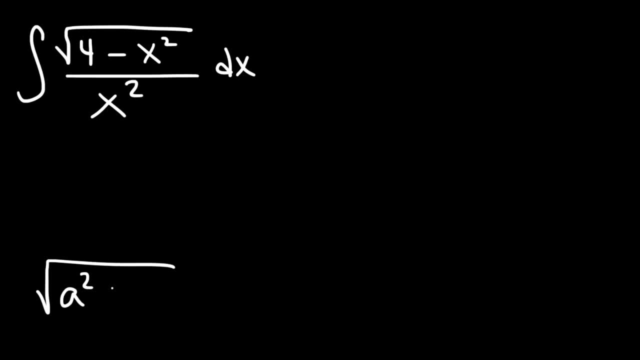 So we can see that we have a problem in this form. And so 4 is equal to a squared. Therefore a is equal to 2.. Now Now x has to be equal to a sine theta. So in this problem, x is 2 sine theta, which means that dx is going to be 2 times the derivative of sine, which is cosine theta, and then d theta. 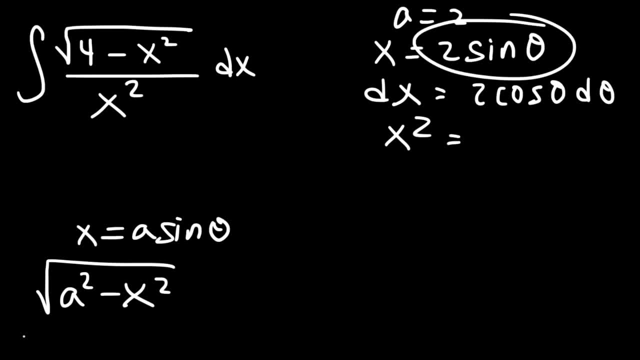 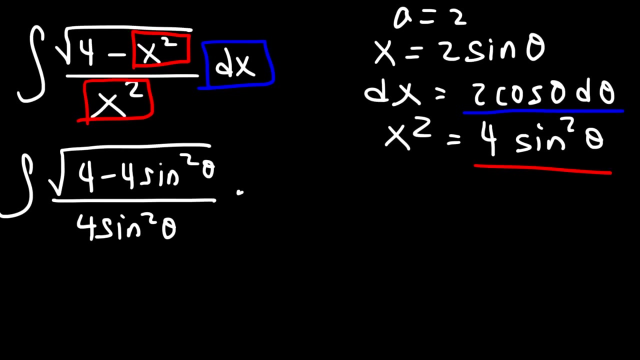 Now x squared is going to be 2 sine theta squared, which is 4 sine squared theta. Now what we're going to do is we're going to replace x squared with 4 sine squared theta And, at the same time, we're going to replace dx with 2 cosine theta d theta. 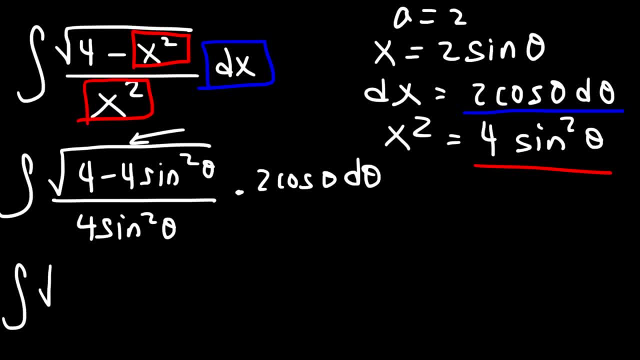 So now, inside the square root, let's take out a 4.. So if we factor out the GCF, we're going to have 1 minus sine squared on the inside. Now I'm going to run out of space, so I'm going to erase everything on top. 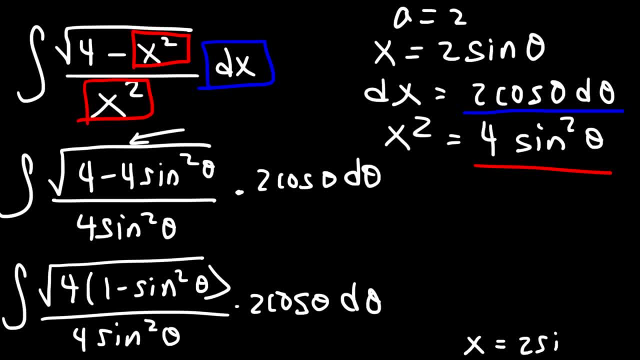 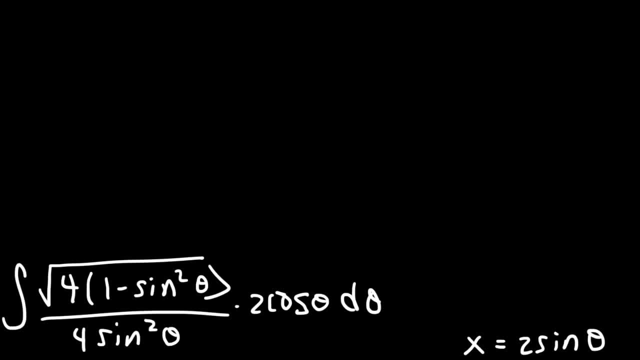 So just keep this in mind: x is equal to 2 sine theta. Now the square root of 4 is 2, so we can take out the 2 from the radical, And 1 minus sine squared is equal to cosine squared. 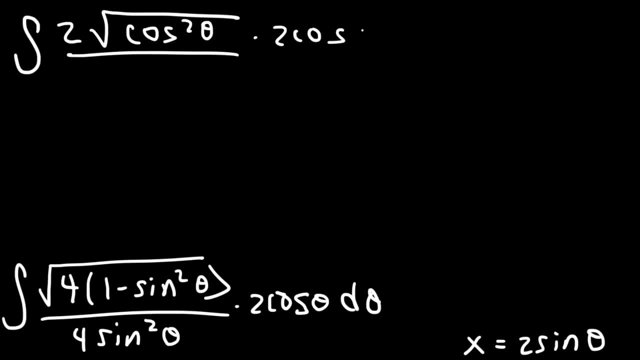 So this is what we now have. In the next step, we can take the square root of cosine squared, And so that's. I didn't want that to happen. That's going to be cosine, And so we're going to have 2 times. 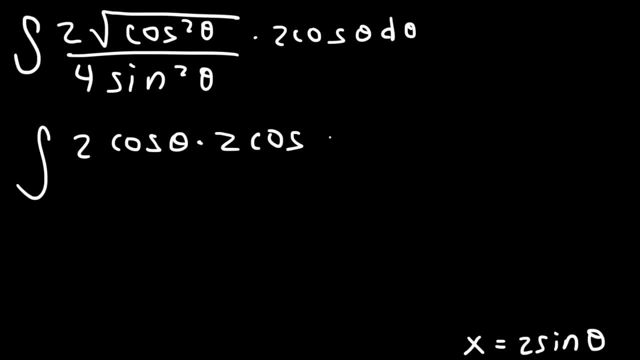 2 times cosine theta times another 2 cosine theta d theta over 4 sine squared theta. Now, 2 times 2 on top is 4, which will cancel with the 4 on the bottom, And so we're left with cosine times cosine, which is cosine squared. 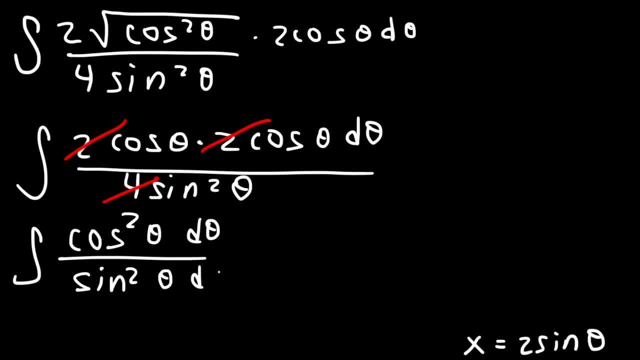 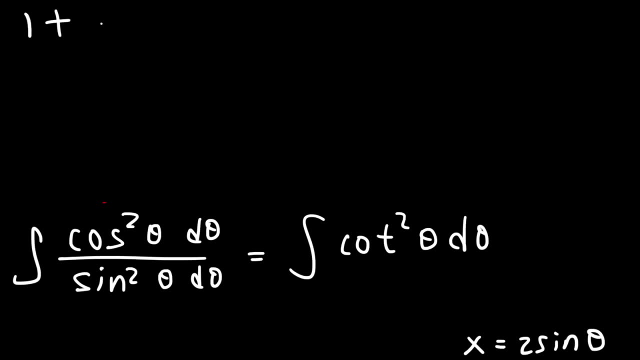 And cosine squared divided by sine squared is cotangent squared. So what do you think we need to do? What do you think we need to do at this point? What's our next step here? Excuse me Now recall that 1 plus tangent squared is secant squared. 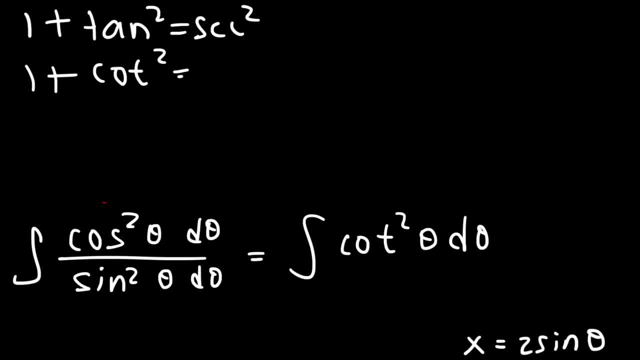 So therefore, 1 plus cotangent squared is cosecant squared. Moving the 1 to the other side, we can replace cotangent squared with cosecant squared minus 1.. And so this is what we now have: The integral of cosecant squared theta. 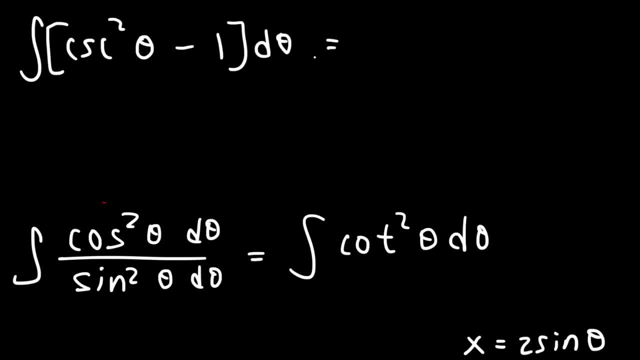 Minus 1, d theta. Now what is the antiderivative of cosecant squared? You need to know that the derivative of cotangent is negative cosecant squared, And so the derivative of negative cotangent is positive cosecant squared. So the antiderivative of positive cosecant squared theta is negative cosecant. 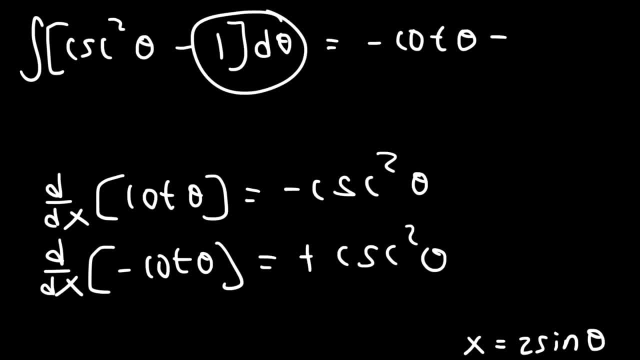 And the integral of negative 1, d theta is simply negative theta. So right now we're getting close, but we don't have the answer quite yet, Even though we've integrated or we found the antiderivative of this expression. 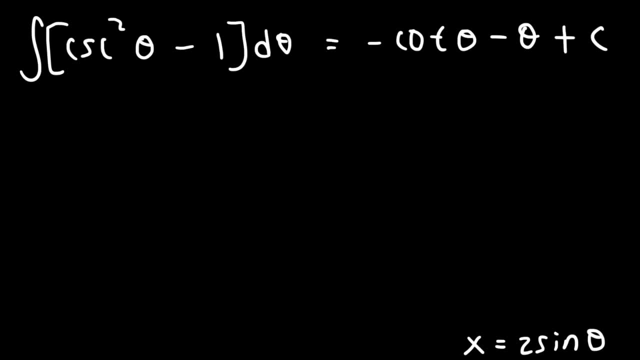 we still need to replace theta with some x variable. As you can see, this is a very long problem. So let's go back to this expression. where x is 2, sine theta, Let's divide by 2.. So sine theta is x over 2.. 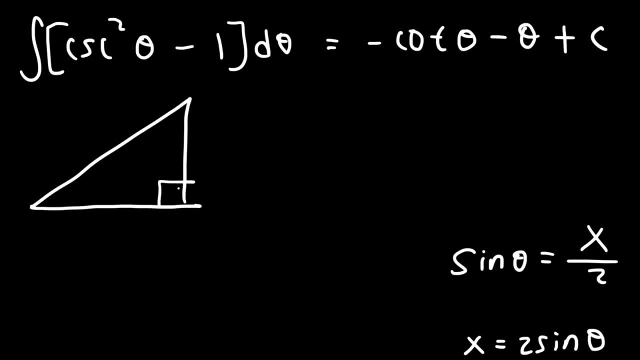 And what we're going to do is we're going to make a right triangle And let's do that a little bit better. And so here's theta Now, based on SOHCAHTOA. we know that sine is equal to the opposite side divided by the hypotenuse. 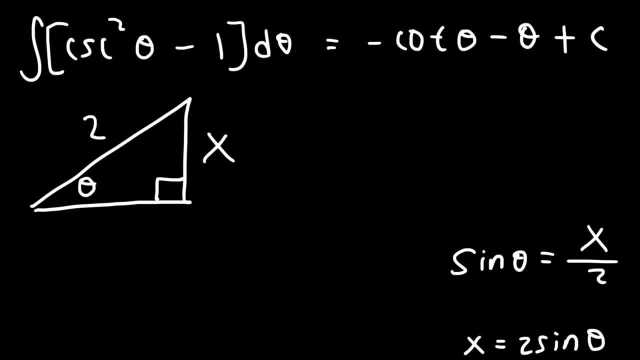 So x goes on the opposite side And 2 is the hypotenuse. Now, using the Pythagorean theorem, we need to find the missing side. So a squared plus b squared is equal to c squared, And let's say a is the missing side. 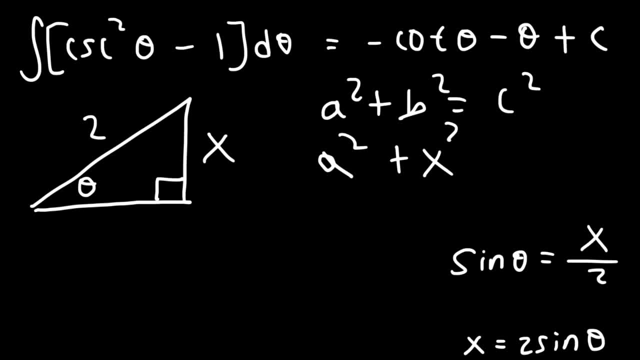 That means b is equal to x. So b squared is x squared, C squared is 2 squared. So moving x squared to the other side, we'll get that a squared is 4 minus x squared And taking the square root of both sides, we can see that the missing side is the square root of 4.. 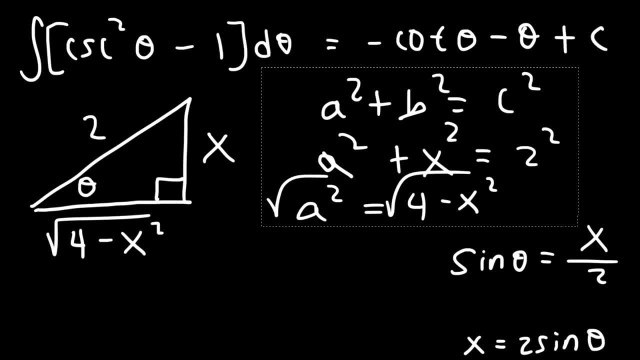 4 minus x squared. So now we can figure out what tangent is Based on SOHCAHTOA. tangent is opposite over adjacent, So it's x over the square root of 4 minus x squared. Cotangent is the reciprocal of tangent.